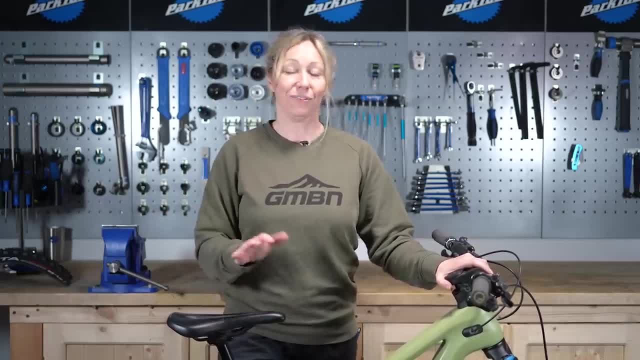 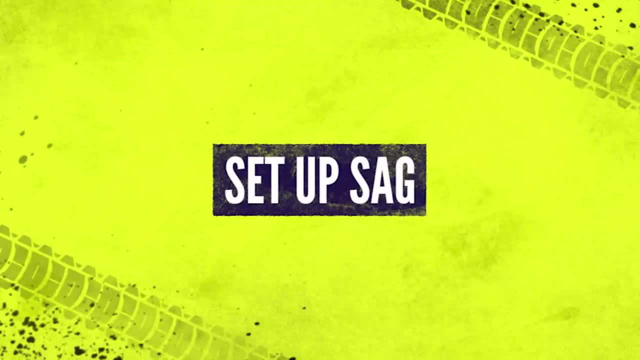 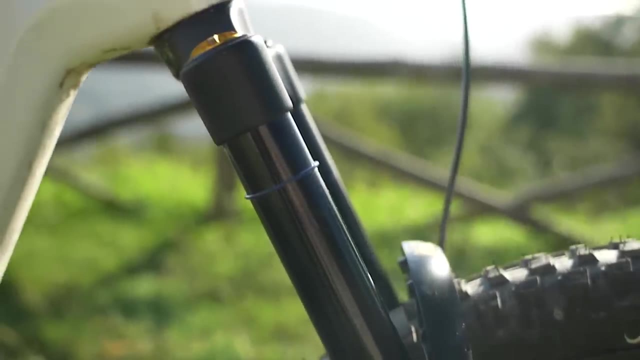 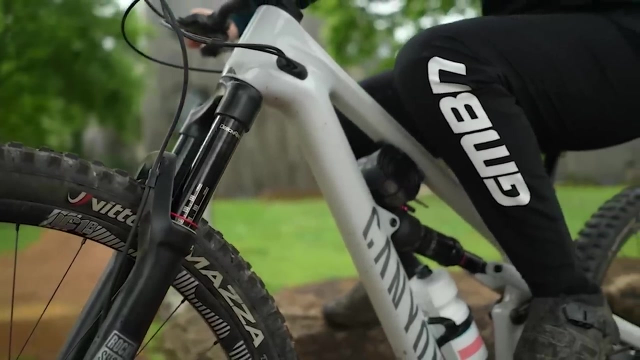 you feel more confident in looking after your bike, and if you can look after your bike, it'll look after you. You don't have to be an expert in setting up suspension or even understand how it works, but setting up your sag is a really good place to start and it makes a big difference. I've seen so. 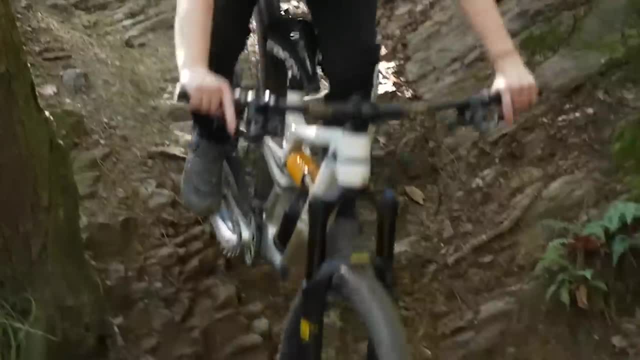 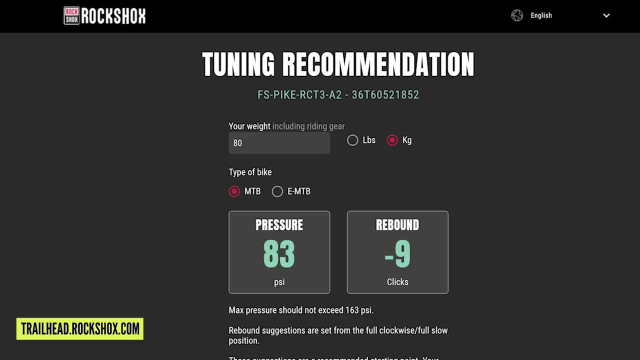 many people with incorrect air pressure, and all this can be solved with just a ruler. Pressure charts on suspension websites are just a guide, and they're a starting place. The only way to know for sure that your sag is set up correctly is to use a ruler. Now, what you need to do is measure the 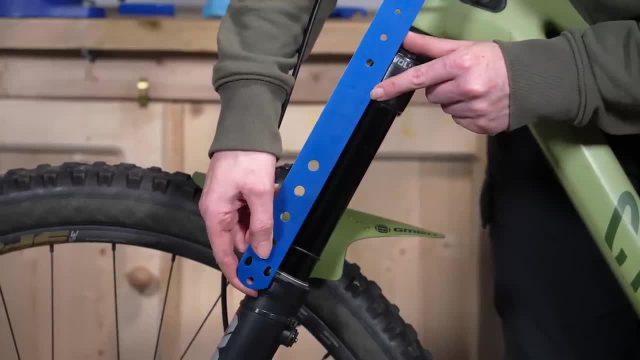 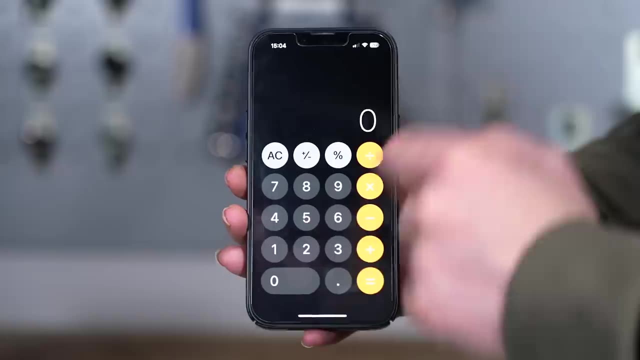 stroke on your rear suspension shocks So you can measure the stroke or the amount of travel on your forks. So with this I've got 170mm forks. That's the total amount of travel. So on a calculator, if we do 170 divided by 100 and times 30, 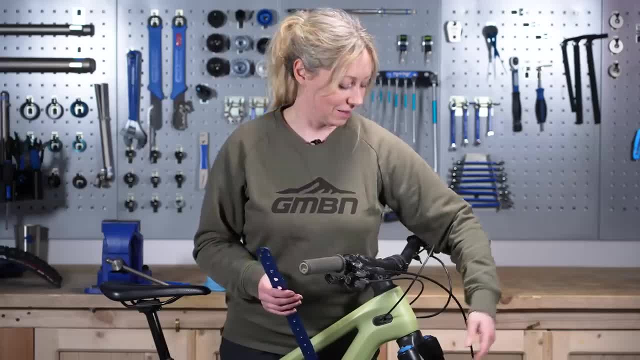 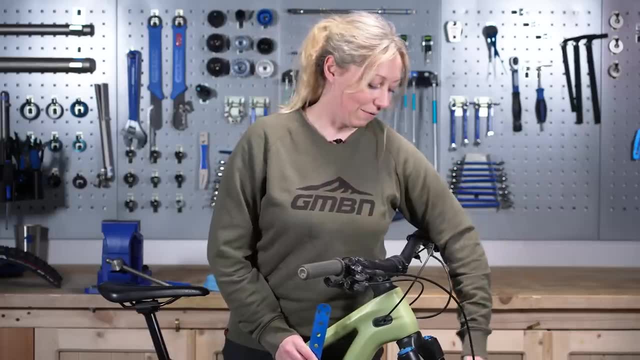 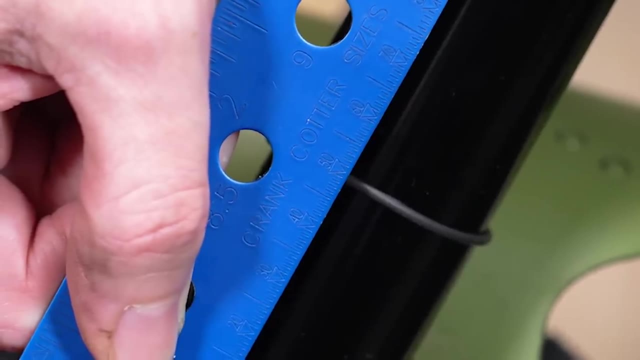 then that lets me know what 30% sag is. So for this it's 51mm. So I know that if I sit on my bike and I get 51mm of movement and my o-ring moves up to 51mm, then I've set my forks at 30% sag. Now, 30% sag is probably a good starting point for. 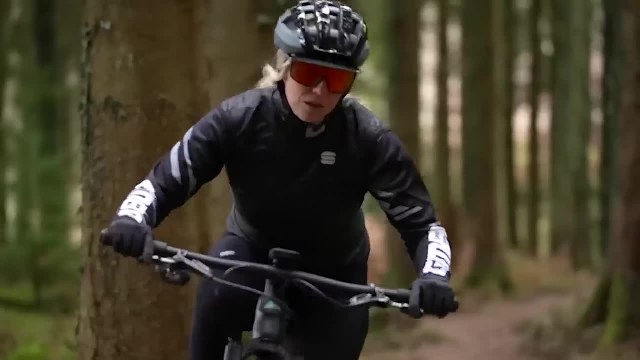 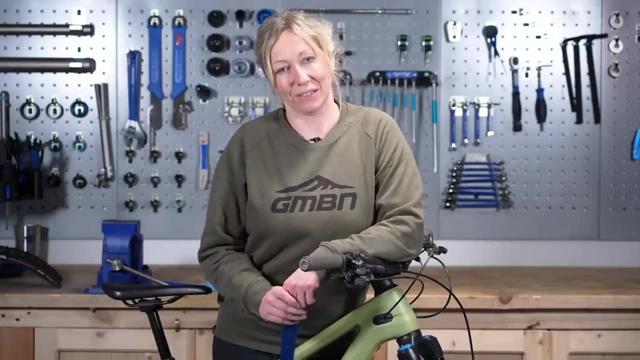 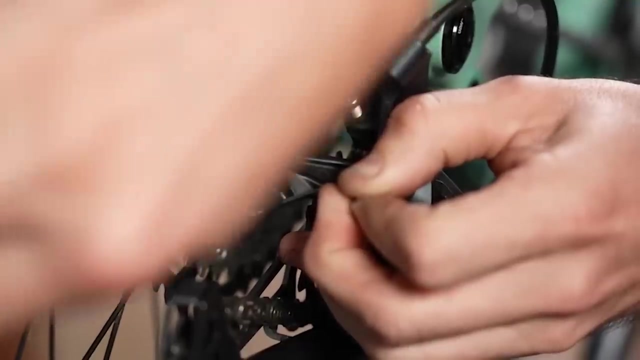 enduro and gravity oriented bikes For cross-country. maybe you want 25%, but these are just base lines and you'll have to muck around with them and see what works for you, Whether you get a local bike shop to refresh your gear cables or if you've done it yourself. 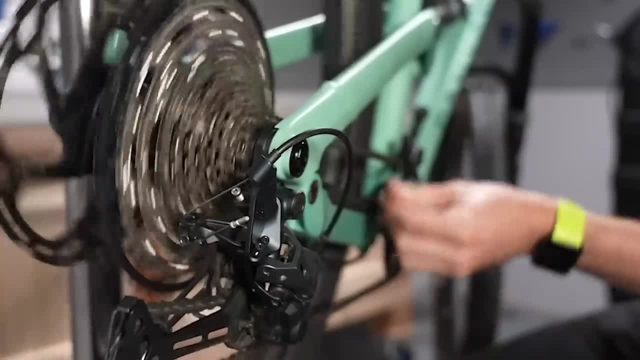 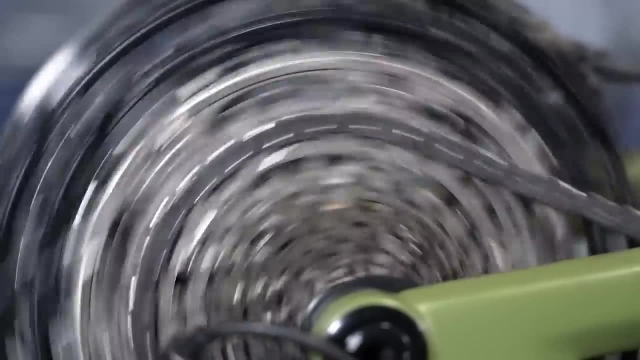 they'll almost certainly work for you. You'll definitely get slack after a few rides and that will cause the gears to skip and crunch. This is totally normal and to be expected with all new gear cables, but you'll need to know how to tighten them back up afterwards. 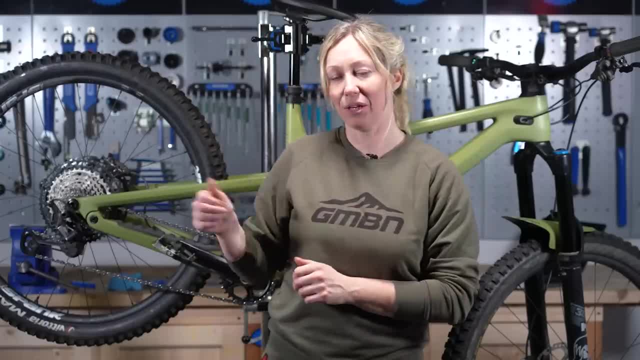 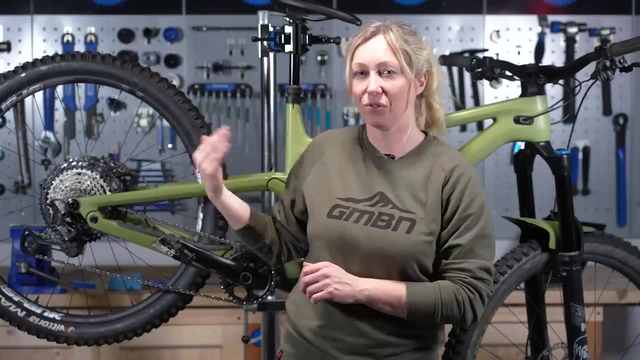 So if you've got new or recent cables and you're trying to shift up into a bigger or an easier gear on the cassette at the rear and it's not going, perhaps it's flicking or it's just not moving at all. there's not enough tension on the derailleur to move it And this isn't a problem with your. 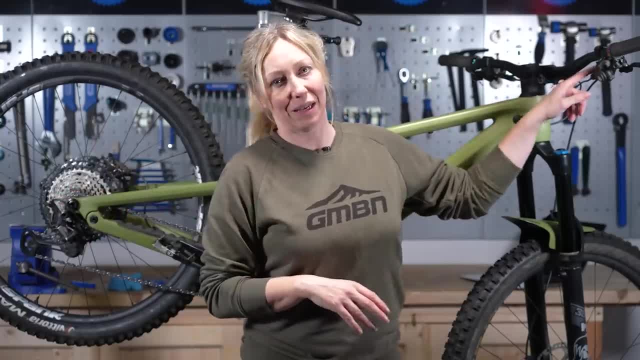 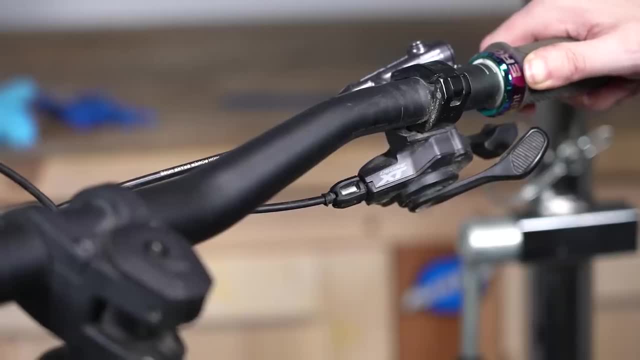 derailleur. You're not going to have to play around with the derailleur. You're not going to have to play with that. You just play with the barrel adjuster up here. So if you're looking directly down at the barrel adjuster, down the shifter, you want to be moving it anti-clockwise, which? 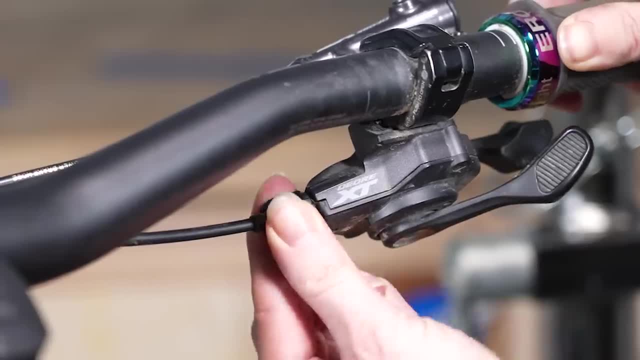 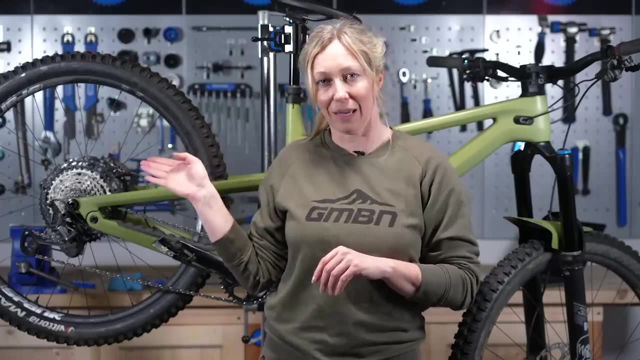 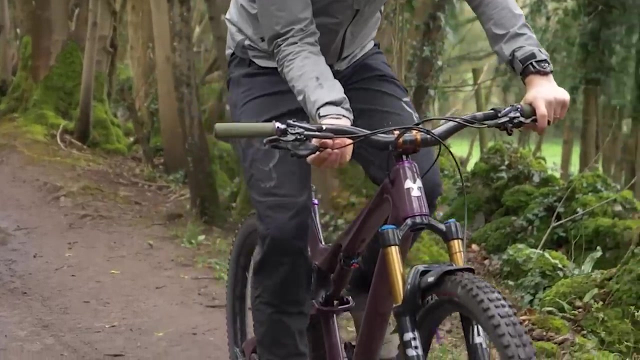 will move the outer cable away from the shifter and it will put tension on that inner cable And that should help you move your gears up into that easier gear. Now tip two is to always do this change while you're pedaling the bike. Now this could be moving it in a stand like I've 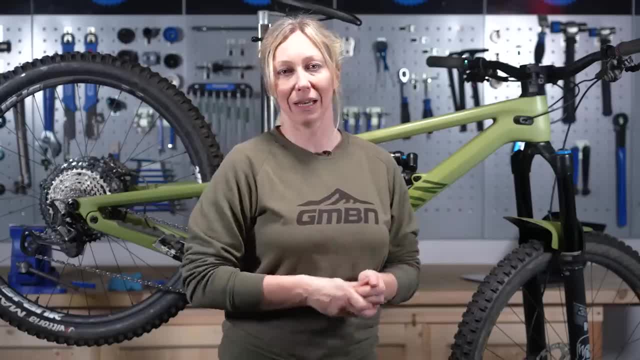 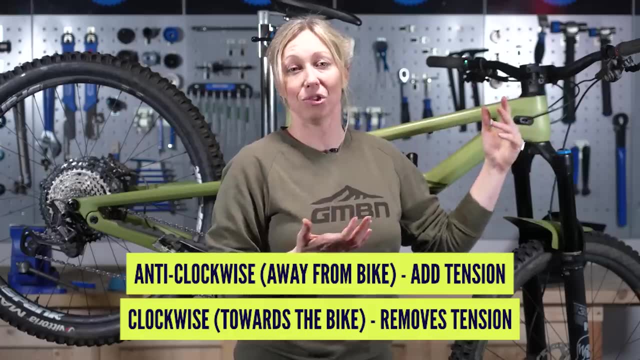 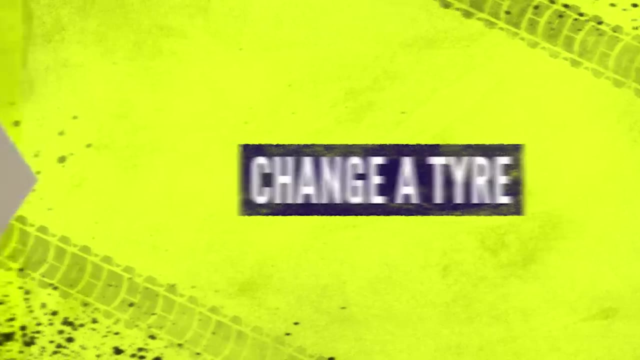 got here, or it could be pedaling the bike out on the street. Make that shift. If it doesn't move, keep adjusting the barrel adjuster anti-clockwise until it does shift and that should solve the problem going forward. We all get punctures and whether you are tubeless or still running tubes, 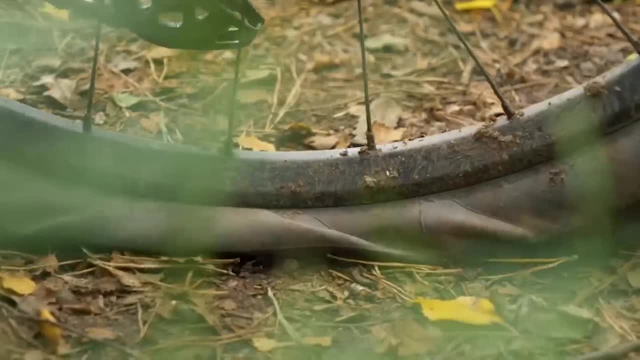 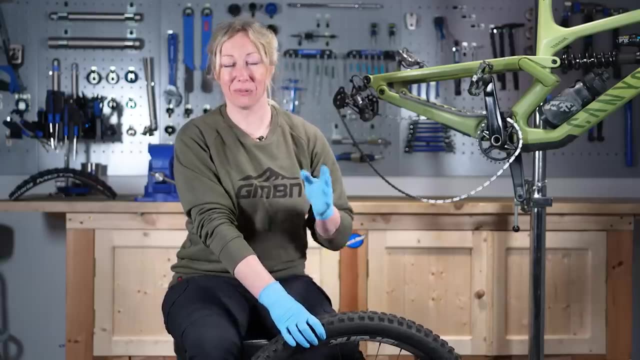 you'll probably need to change a tire at some point. I've heard some horror stories before, but I swear most of these problems can be solved if you tick off the following tips. My first big tip to remove a tire is to make sure there's no more air in there at all. This will make it easier to manipulate. 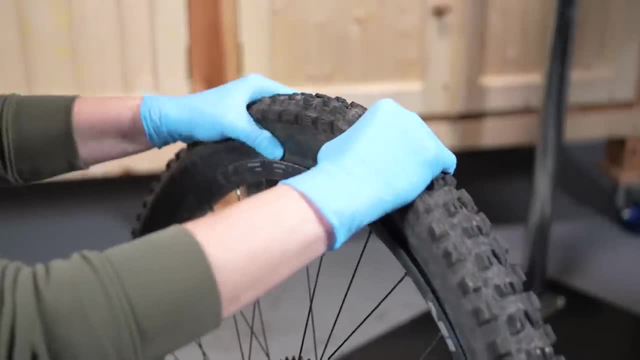 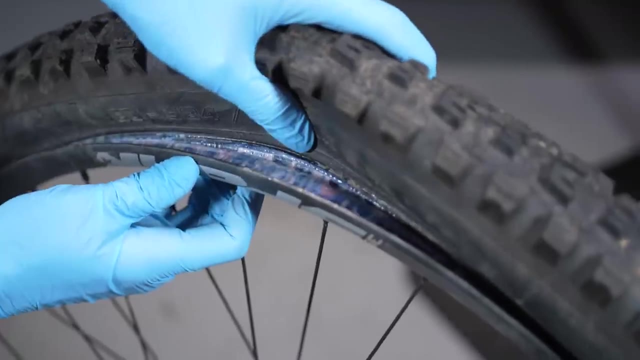 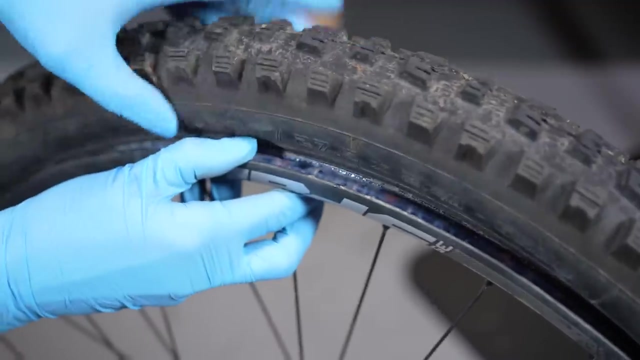 And then my next tip is to move it off the shoulder of the rim. break the bead off and move it into the central channel of the rim. This central channel will have a slightly smaller diameter than the shelf of the rim, and this will leave your tire feeling a little baggier and much easier to get a tire lever into. 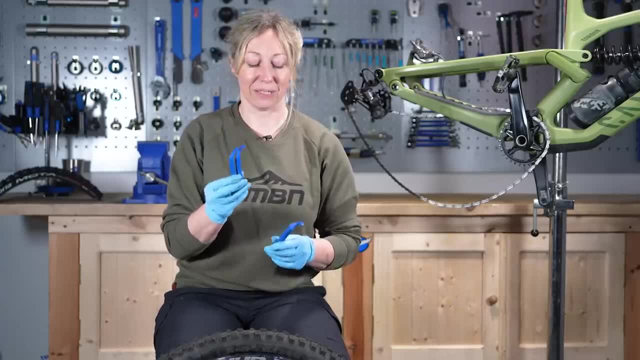 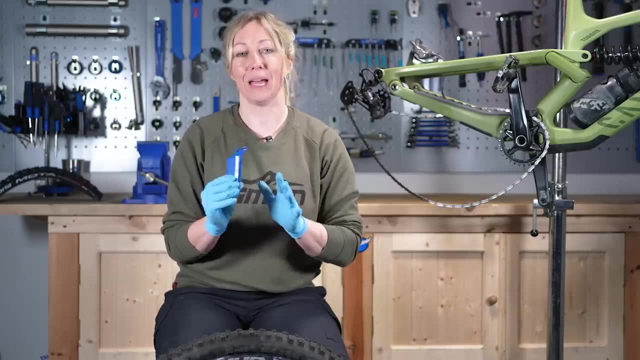 My next big tip is to have at least two levers. better to have three as well. And definitely you want some nylon or plastic levers, not metallic, because they will damage your rims, So make sure they're softer than your actual rim material. 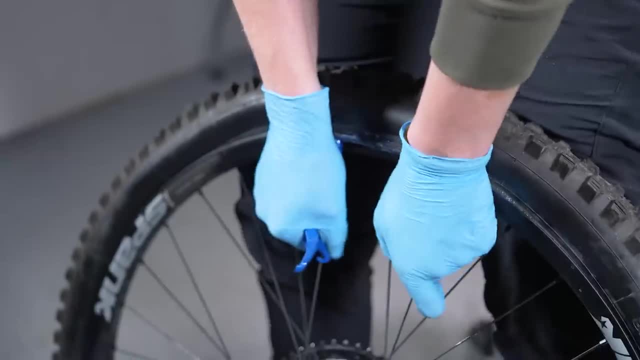 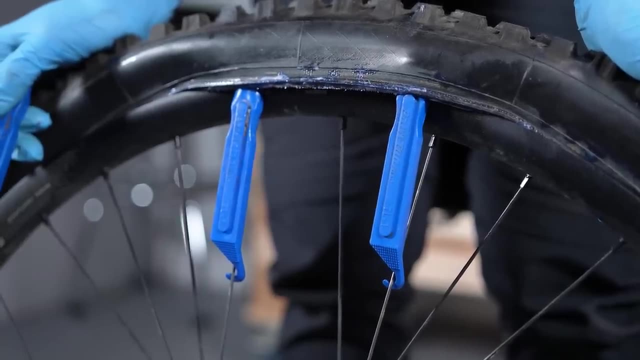 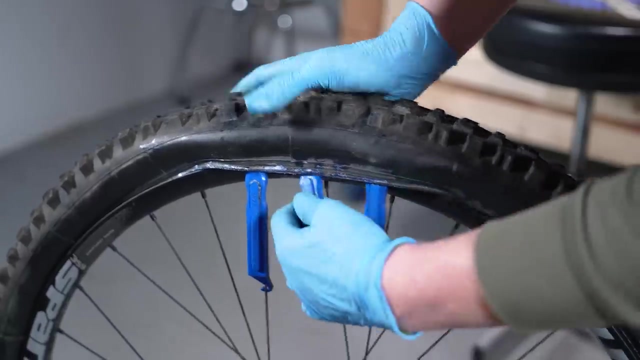 And also, if you can get hooks on the end, then these go a long way to holding the tire over the rim and hooking into your spokes, And that way you can use two on either side hooked over onto your spokes, And then you can even use a third one in the center to leverage it out. 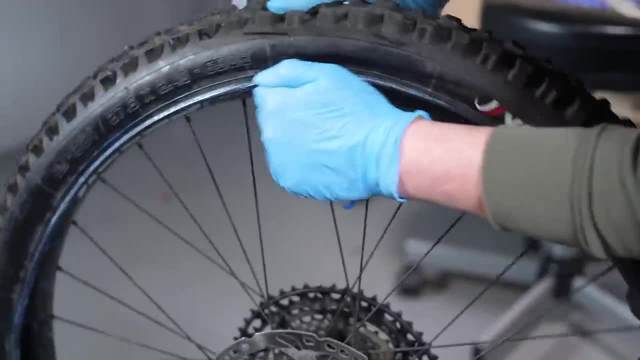 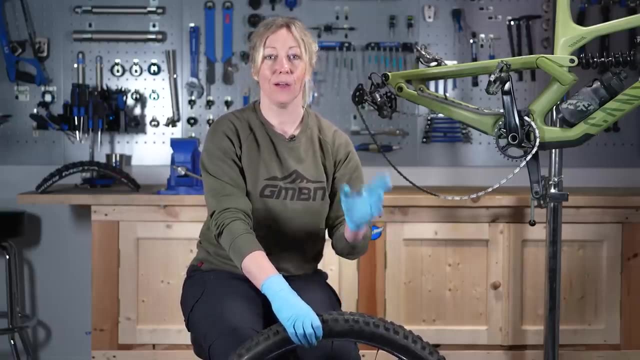 and rotate it all the way around the rim to get it off. Now, once you've done your repair, or put your inner tube in. a similar principle applies to earlier, where it makes things a lot easier if you can get the bead of that tire into the center of the rim. 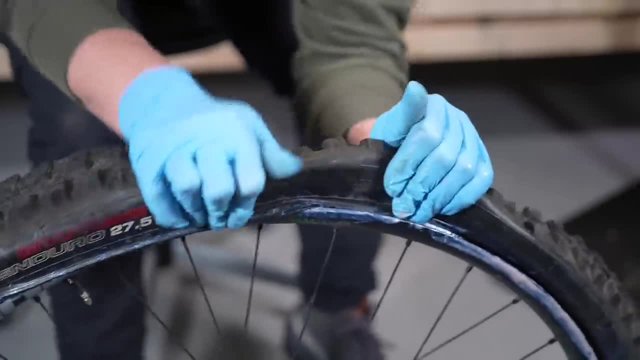 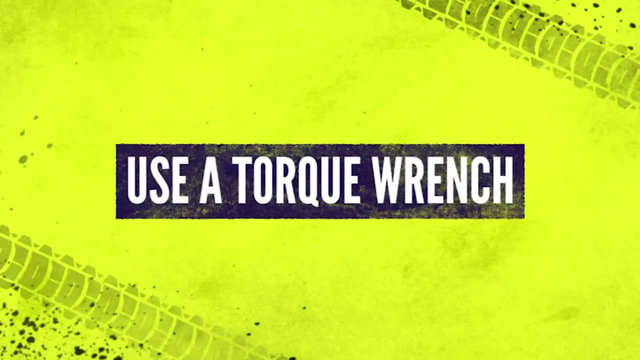 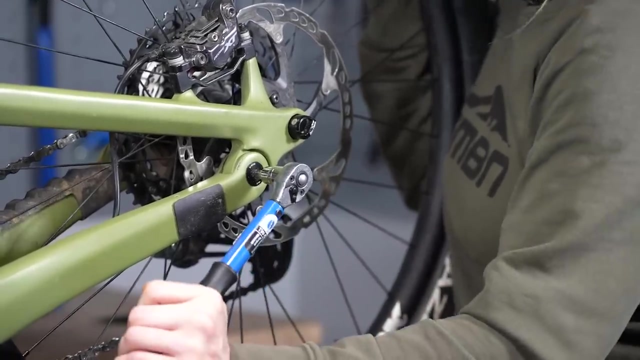 And that means it won't be so tight when you chase it back round. You should be good to go. We might have a question. here mentioned torquing up bolts a lot, but what does that actually mean? Now? a torque wrench basically controls the amount of leverage you push through a bolt, because if you over tighten, something like 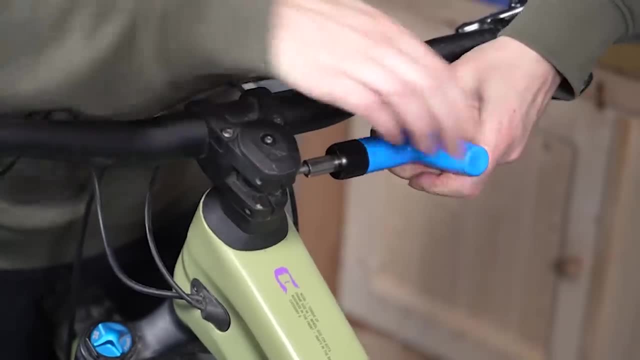 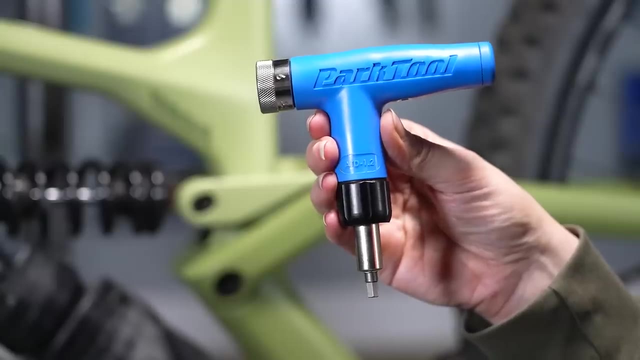 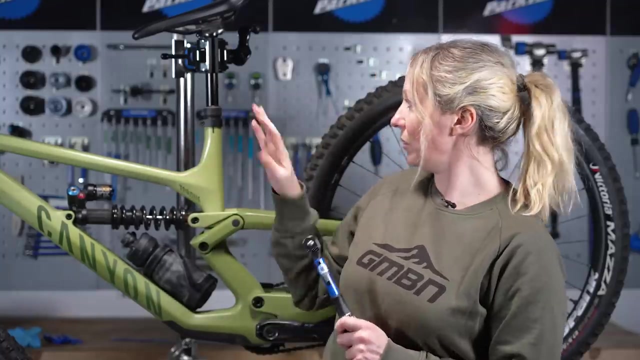 a stem or a brake on the handlebars, you could potentially crack the component it is clamping to, or you could round the bolt or even strip a thread. so these are very handy devices to have. So every bolt on every part of your bike will probably have a different torque setting. you'll know because it 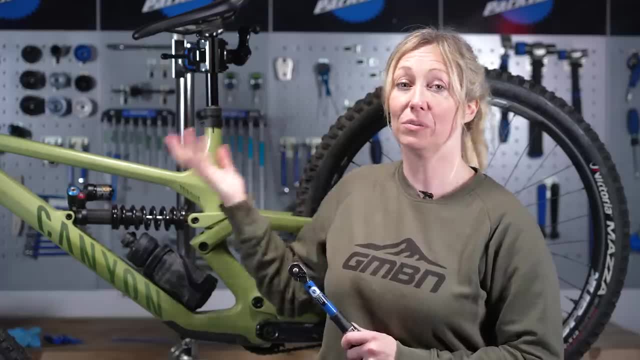 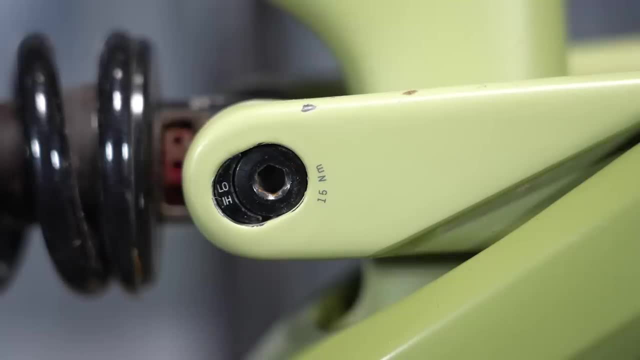 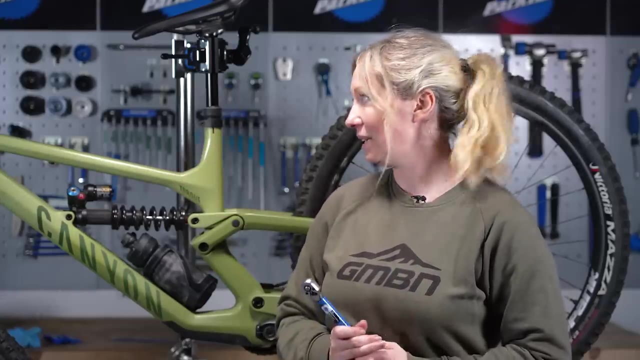 has a number followed by nm, which means newton meters. so I've got a six newton meters written on the part up here. I've even got 15 newton meters written down here and if any of the bolts don't have any writing on them, then do check a website or the manual for your parts to see what the torque 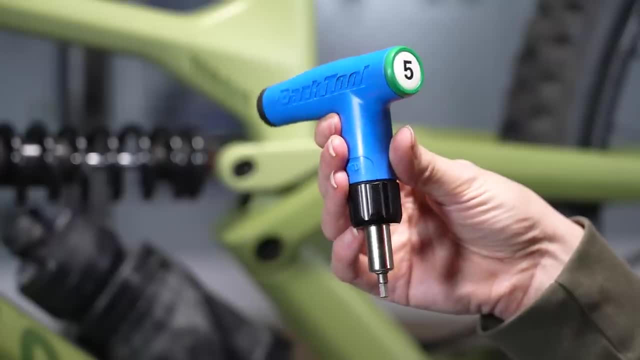 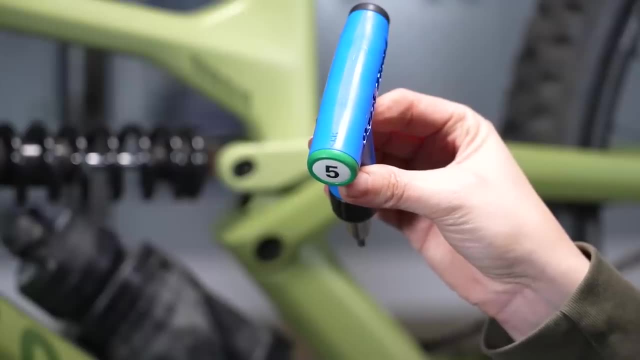 setting is for that. So something like this preset torque driver only has one setting. so, as you can see, it's got a big five on there and that is five newton meters, so it'll click as soon as it will get to the torque setting. So if you want to check that out, you can do that by clicking on the. 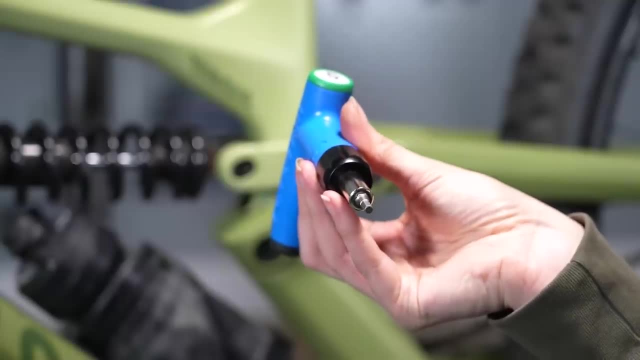 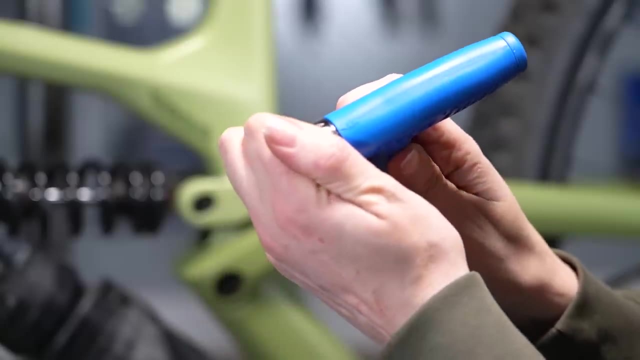 button at the top of your bike and you can see that the torque setting is set to five newton meters and it won't let you tighten anything beyond that. So for a bike, I think it's good to get an adjustable one like this, where you can rotate the dial to the appropriate newton meters, so we can 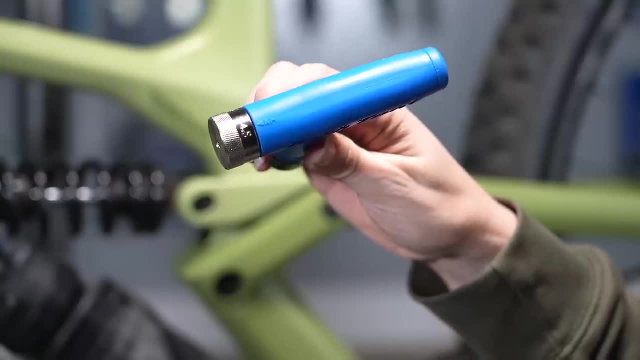 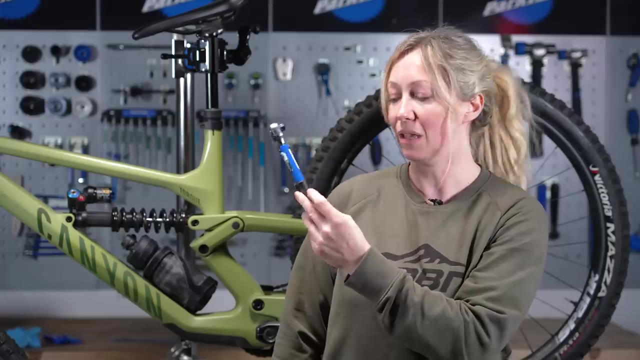 choose four or five or six on this one. Alternatively, you might see these ones are more popular, and this will allow you to go down to decimals of newton meters as well. Now all you have to do is dial the bottom in order to get your correct torque setting in the 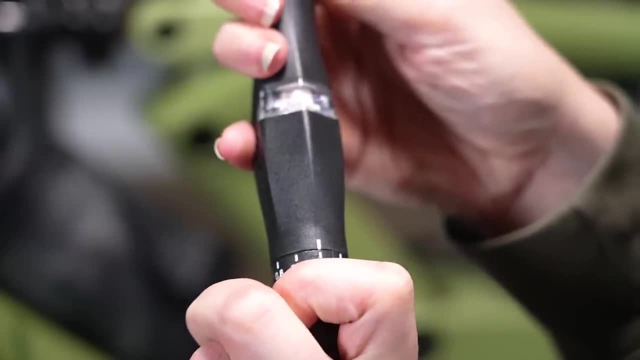 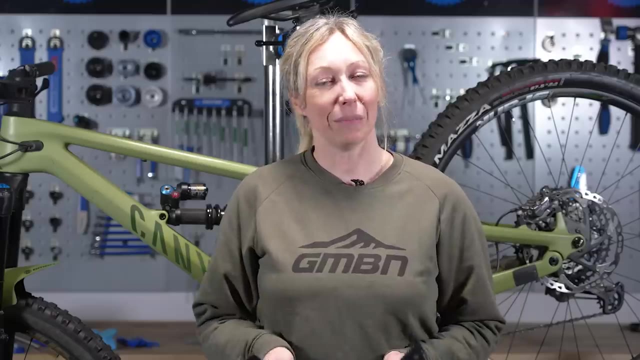 window, and then you also have some extra adjustment to get 0.5, 0.8 and different decimal versions of that newton meters as well. Bonus tip for you: if you're talking things up correctly and you still feel like parts are slipping, then you may need to use an assembly. 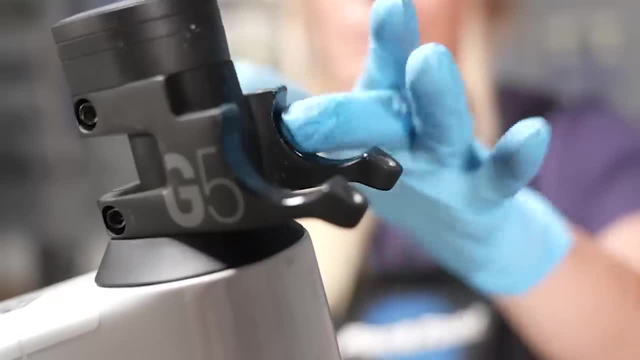 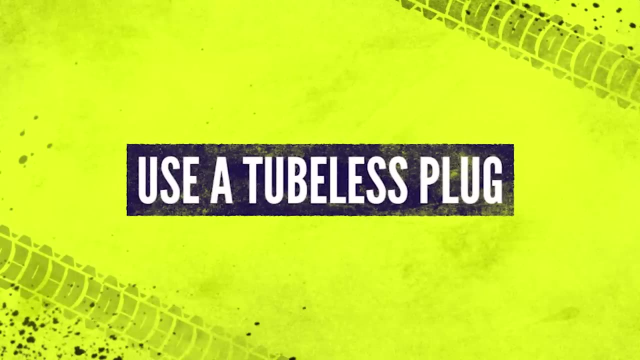 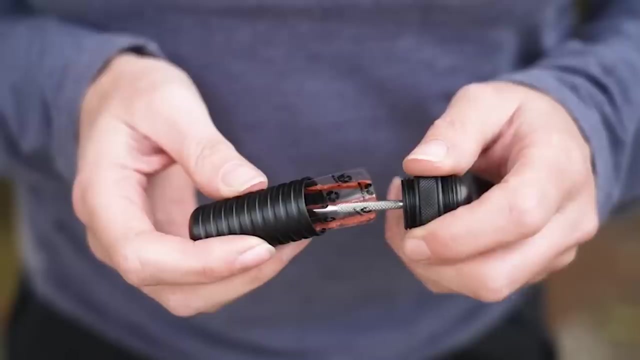 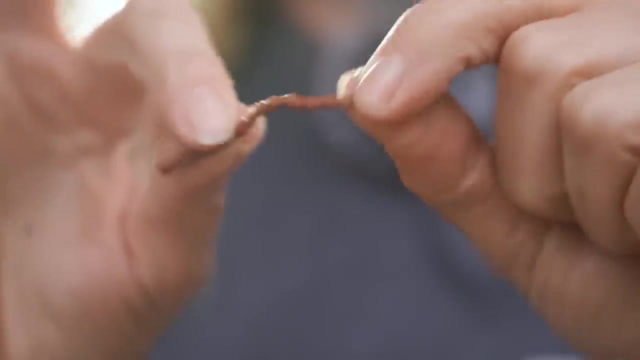 grease or something like a max grip carbon paste, because this has grit in it and it'll take up the imperfections and help you torque things correctly. Tubeless tire plugs are brilliant inventions. They mean that we can often fix a puncture without taking the wheel off the bike or even the tire off of the rim. Now my big tip for you. 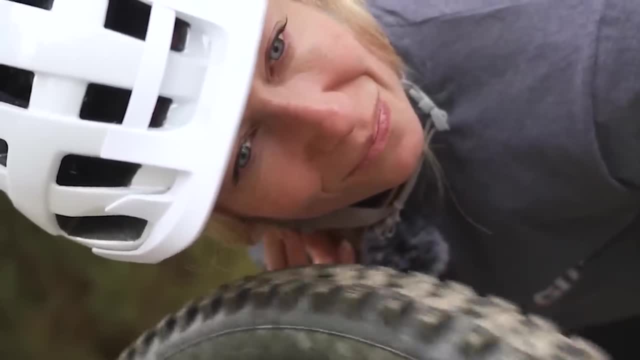 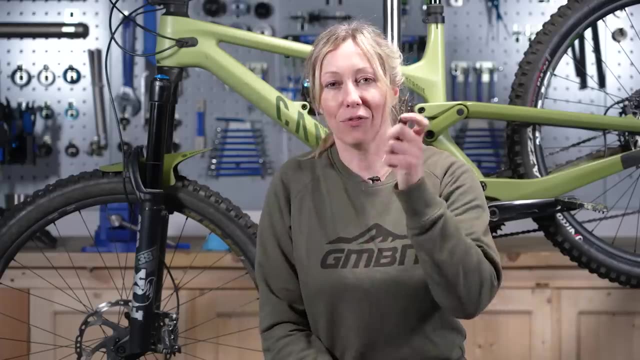 is to find the hole by using your ear and the side of your cheek and move that wheel around so that you can hear and feel the air, and then you'll find the hole and be able to plug it. My second big tip is to make sure you push it in gently and then you'll be able to plug it in. So if you're 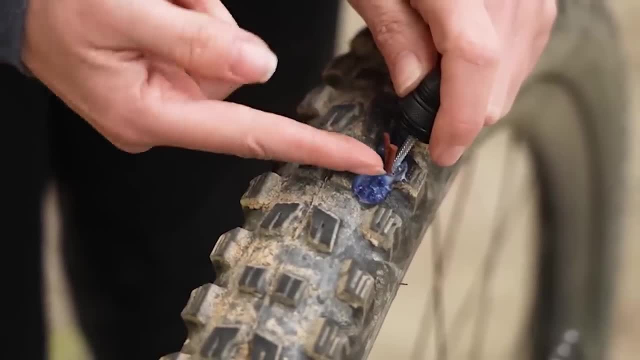 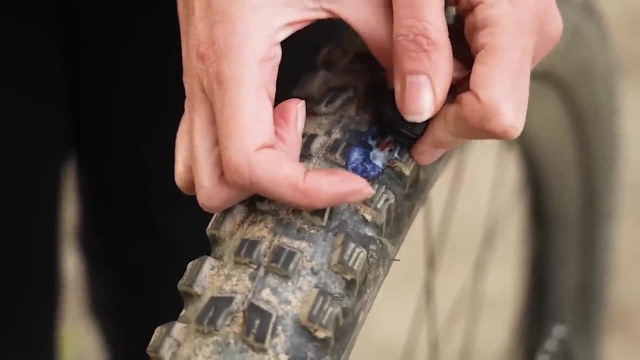 using a flat tire. you want to push it in so that there's two halves either side of your plug and then it'll fold in place and give you double the amount of plug in that hole. and you want to push it gently in enough that the end is just poking out Enough so that it doesn't go into. 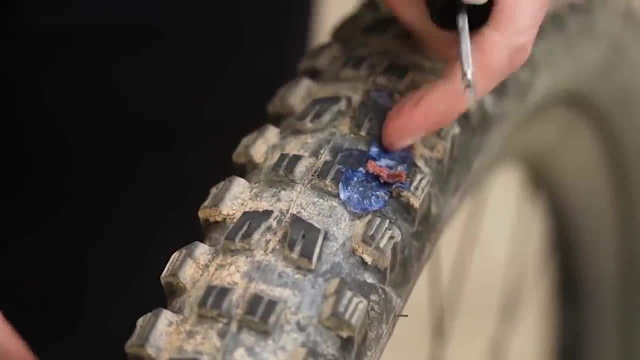 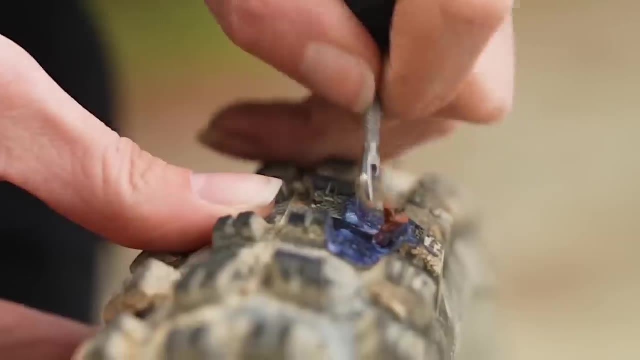 your tire. but also you don't want too much sticking out of the tire as the trail might rip it out along your way. Bonus tip for you here: if you have the time, a little bit of puncture repair glue will help you out a little bit. If you don't have the time, you can use a little bit of. 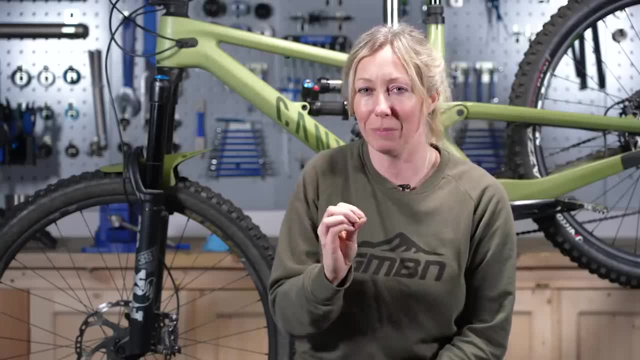 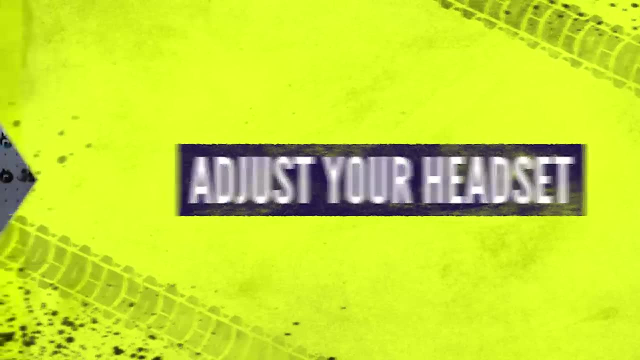 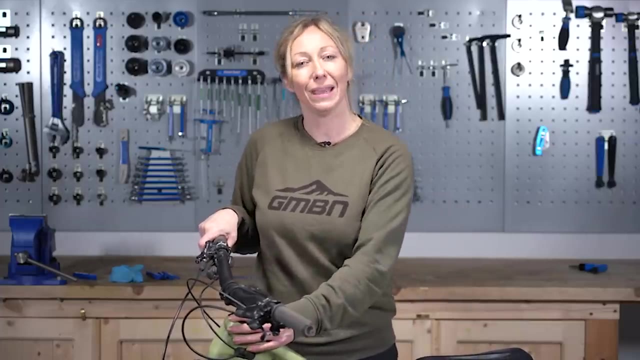 tape around the edges, we'll seal it in on a more permanent basis and it'll make it a lot more secure. A loose headset is actually really common, but it's one of the simplest things to fix. so if you feel a knocking in the front of your bike- perhaps a rattle, or maybe your bike's even juddering when, 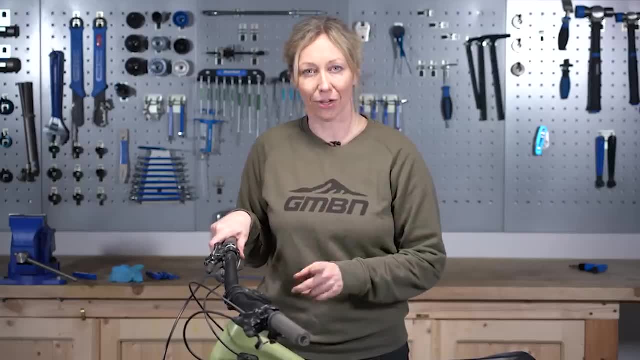 you apply the front brake down a hill, that's probably a loose headset and the way to know for sure is to apply the front brake to a single flat tire and the bike. if you feel the bump or anything around the edges will seal it in on a more permanent basis and it will make it a lot more secure. 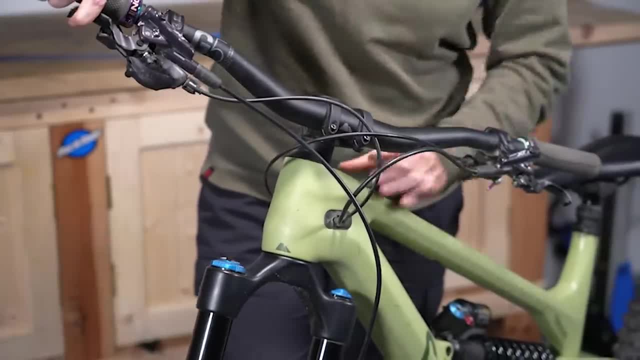 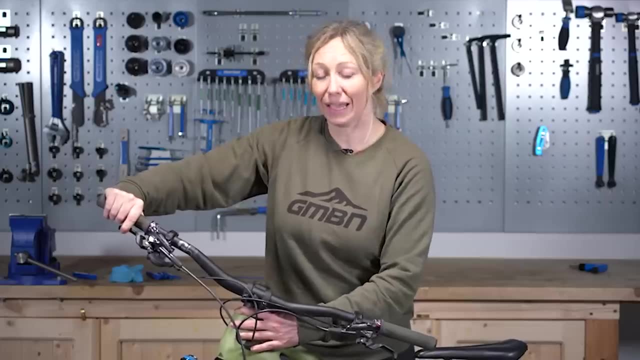 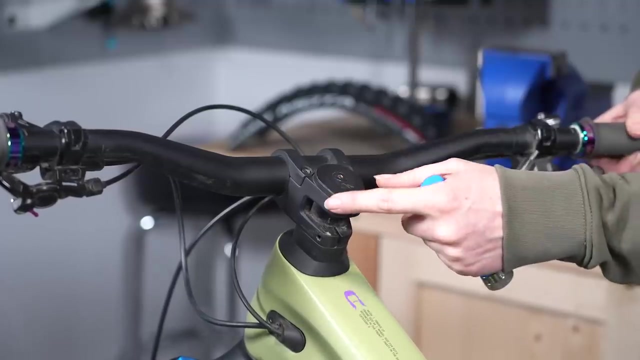 is to apply the front brake, turn the handlebars and then get your hands around the headset area and give it a good rock. now i can feel a knocking and i can even hear it there, so i know that headset is loose. now this is the bowl that is compressing your headset. but what you need to do 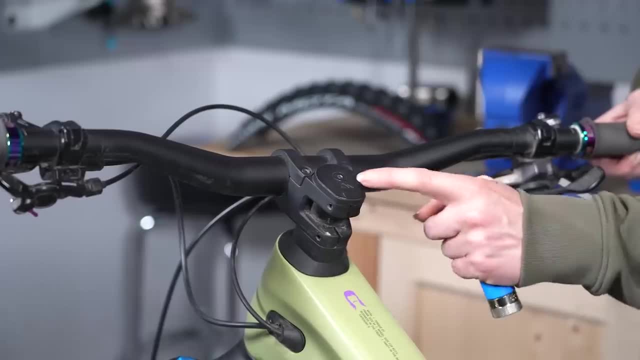 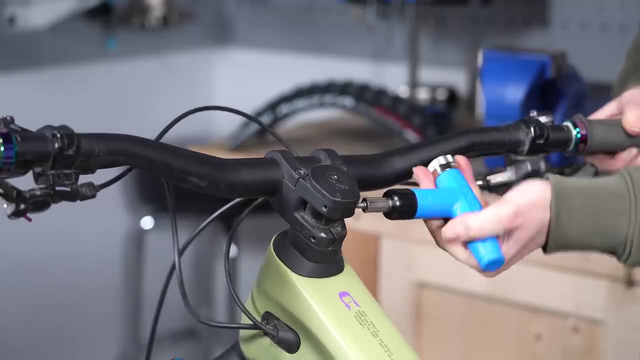 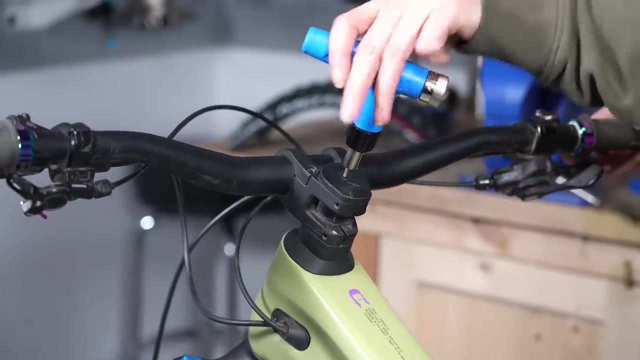 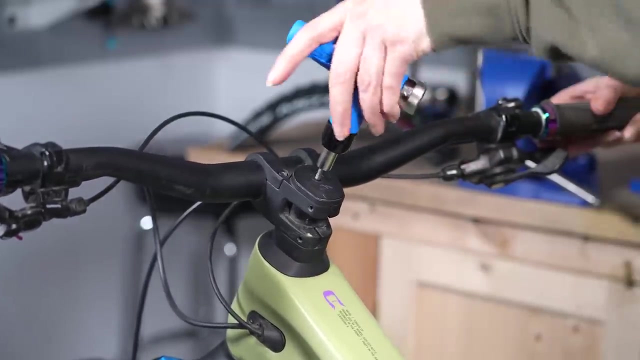 is release the tension on your stem first, otherwise we'll be just tightening this bolt into the stem. so first loosen off the bolts on your stem and then we can tighten up this bolt, and we just do it by hand until that rattling has stopped. if you tighten it too much you could end up pulling the star nut from the fork steerer tube. 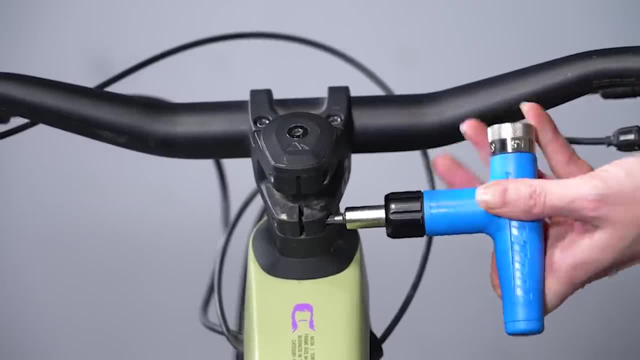 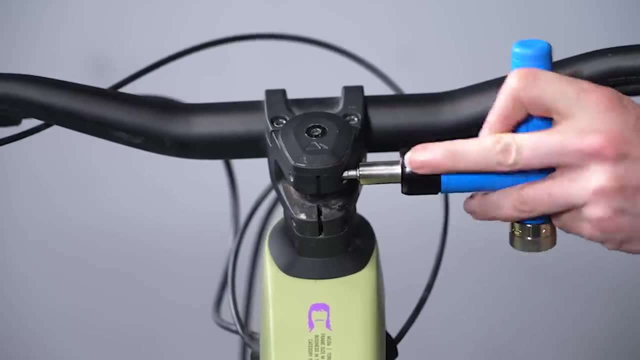 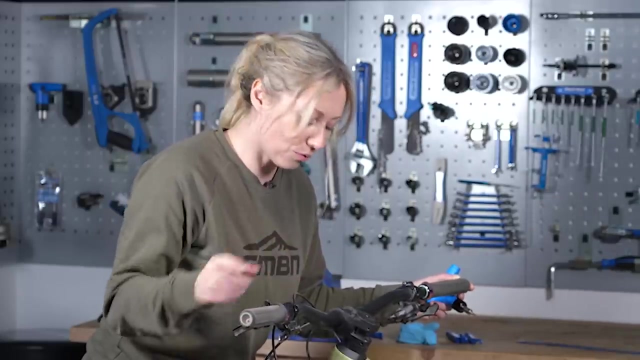 out completely. once you've tightened that up, you can go ahead and tighten up your stem bolt into the stem. so first loosen off the bolts on your stem, as this is simply just clamping around the steerer tube in order to stop that from rotating. bonus tip: here: i like to line up the handlebars with my fork crown to ensure that my steering 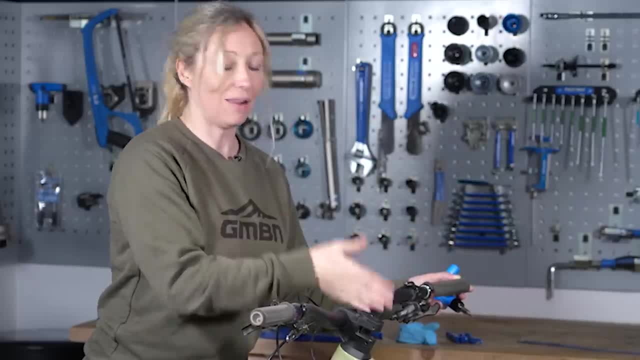 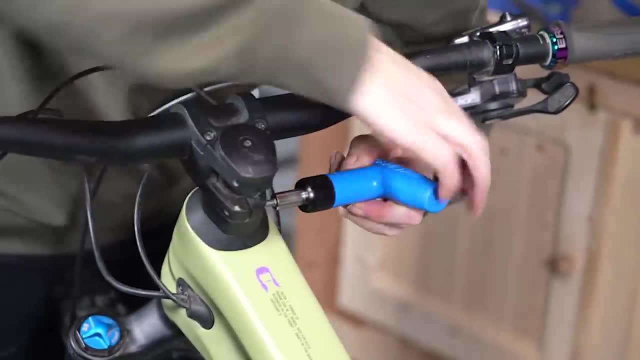 is really straight, but you can stand the other side and line up your stem with your tire if you want. and finally, if you've tightened this all up and you still think your headset is loose, it could be another thing. try undoing the top bolt and having a look at how much. 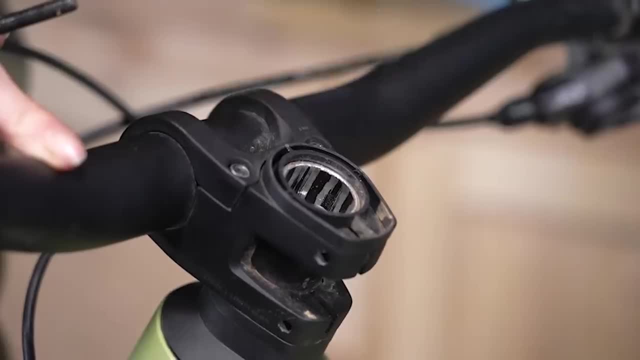 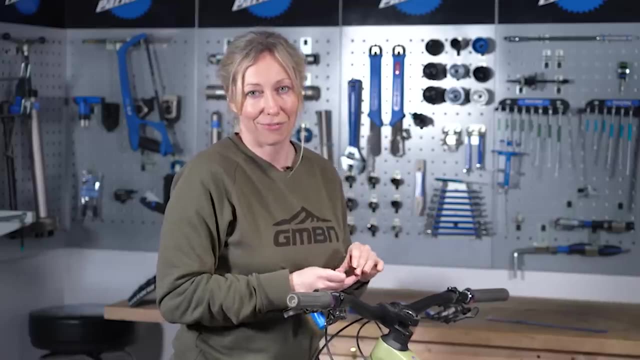 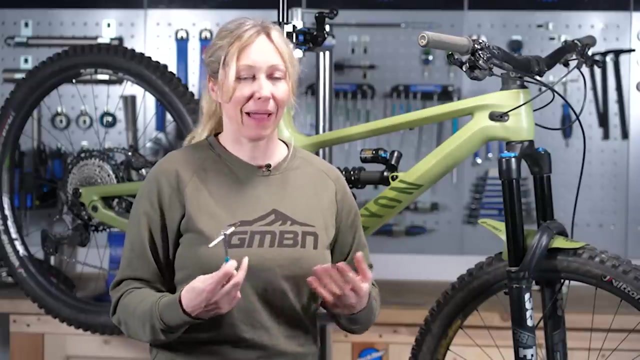 gap there is between the steerer and the top of the spacer or the top of the stem. there should be three to four mil difference in order to compress the headset enough. if your brakes are really noisy, perhaps they feel quite draggy. or if you spin your wheel and they 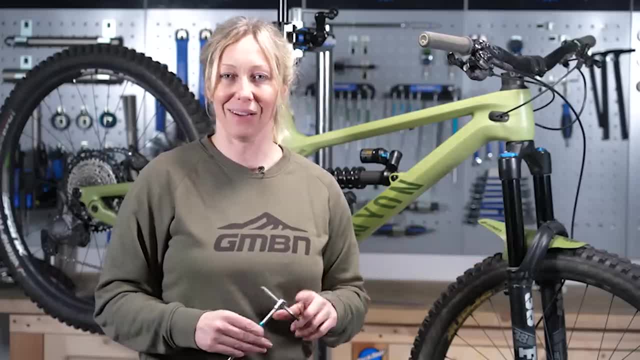 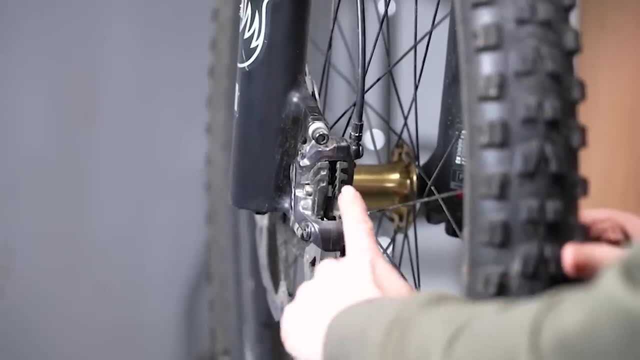 come to an abrupt stop. chances are you need to realign your caliper now. that sounds really scary, but it's actually really simple. so thanks for watching and, as always, stay safe and never let your loudspeaker pick you up. this noise here is the disc rubbing on the left hand side of the pads, and that just means that. 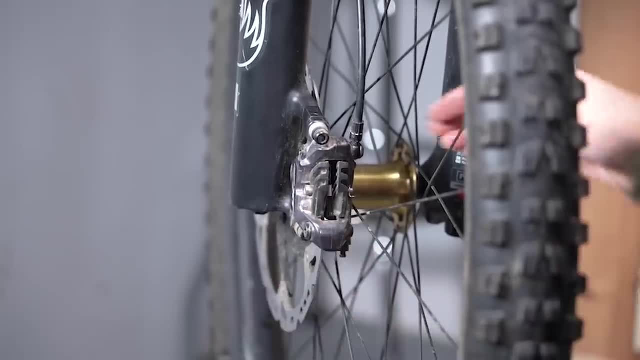 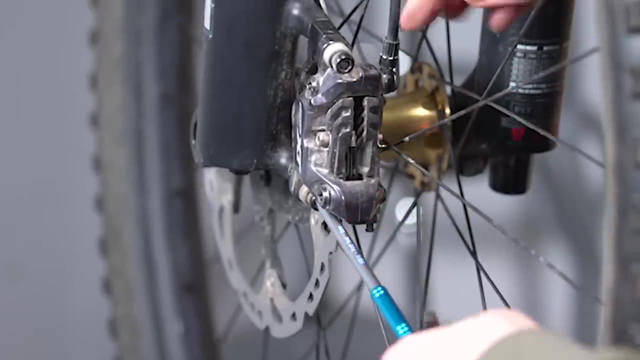 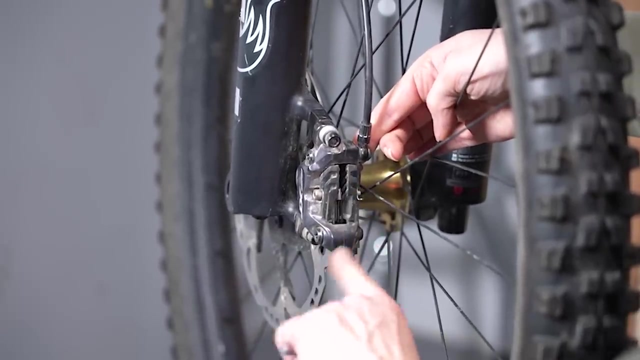 this caliper is not central around the disc and all we need to do is loosen off both bolts for this caliper and we can see that this caliper is now loose to move. so we can move that and make sure that the disc is now central. so, with all your fingers out the way of the disc and the tire.